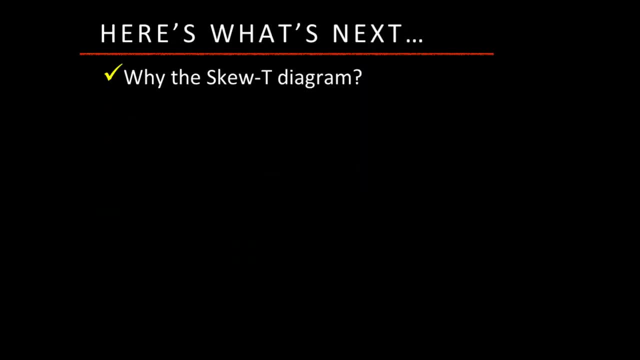 So today we're going to talk about why use a SKU T-LogP diagram. What's the purpose? Why use this diagram in your pre-flight briefing? The next, we're going to get into the components of a SKU T-LogP diagram. 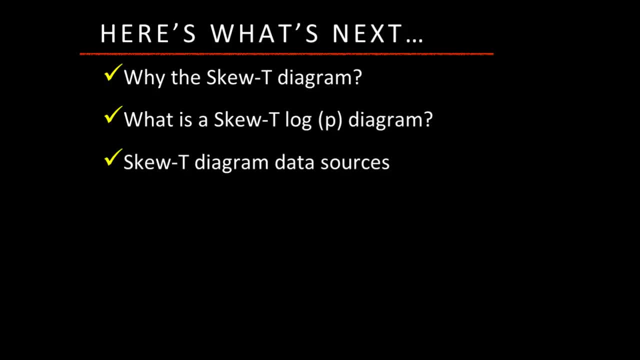 And we'll go through and talk about the input data sources that are used for the SKU T-LogP diagram And again we'll cover some of the various different lines on the SKU T-LogP diagram and talk about the base diagram itself. 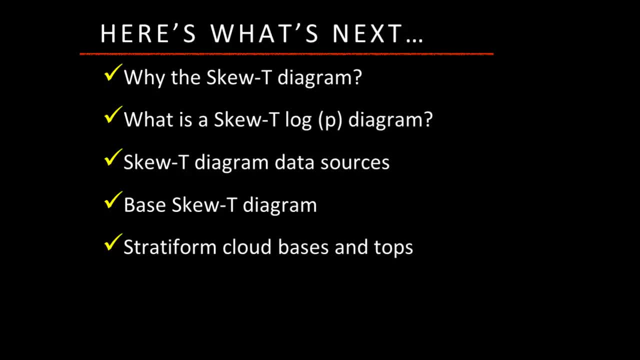 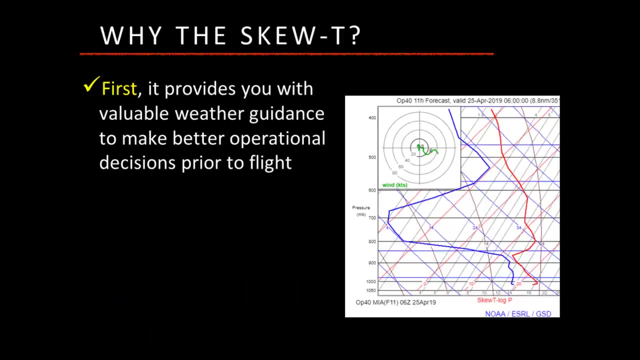 And then go into some application of how to determine stratiform cloud bases and tops, look at freezing level and icing and at the end, if there's time, we'll have some questions and answers. So why the SKU T-LogP diagram? 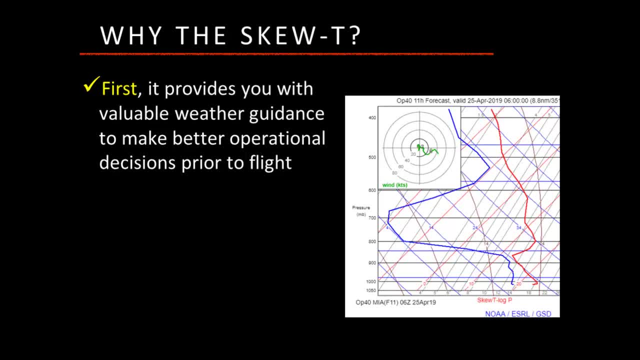 Well, first, it provides you with a lot of good weather guidance to help you make those operational decisions prior to flight, And I think it really covers and increases your situational, Your situational awareness, makes you more aware of what's going on, because it really fills in those gaps and it confirms or even potentially contradicts other guidance you might be using. 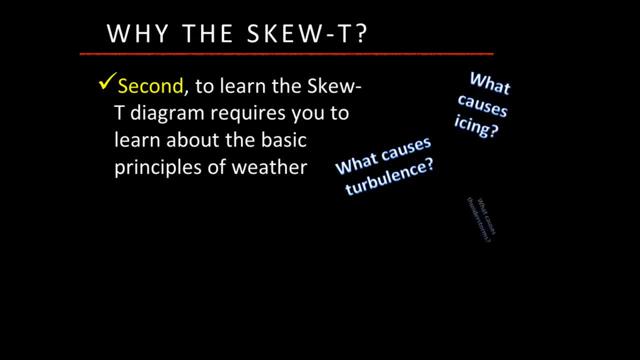 And second, to learn the diagram really requires you to learn the basic principles of weather. What causes icing, turbulence, thunderstorms, What causes that low-level wind, shear or mountain waves? All those elements really provide an added advantage to learning this diagram. 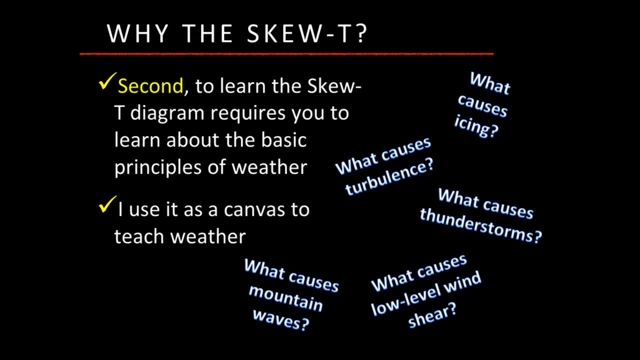 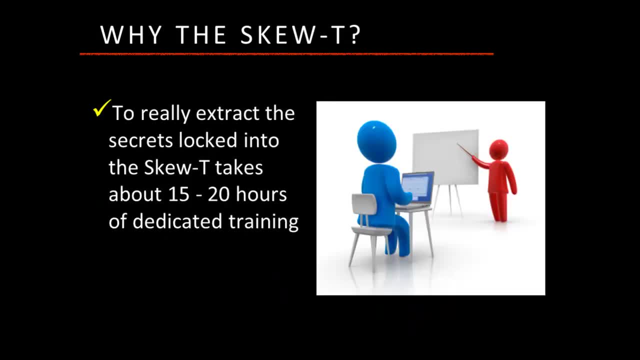 And the second is that it actually uses a canvas to teach weather. So when I'm teaching the pilot about the SKU T-LogP diagram, well, I'm actually teaching them all about weather. So one of the questions I get is: Scott, how long is it going to take me to learn how to use this diagram and become really proficient at it? 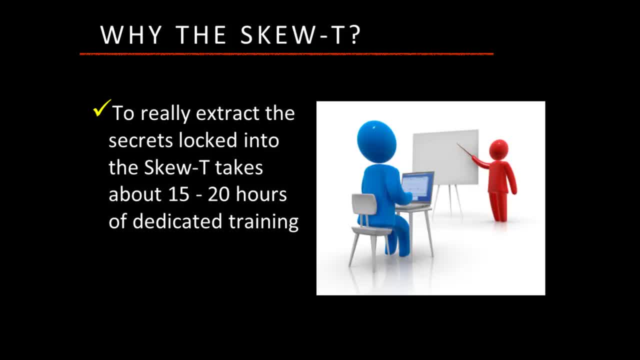 Well, I generally say it's around 15 to 20 hours or so of dedicated training. I've done this with a number of pilots and it's worked out real well, Right? Yes, So over a period of 15 to 20 hours, that's a long time. So over a period of 15 to 20 hours, that's a long time, Right? So over a period of 15 to 20 hours, that's a long time. Yeah, Right, Yeah, Yeah, Yeah, Yeah Yeah. 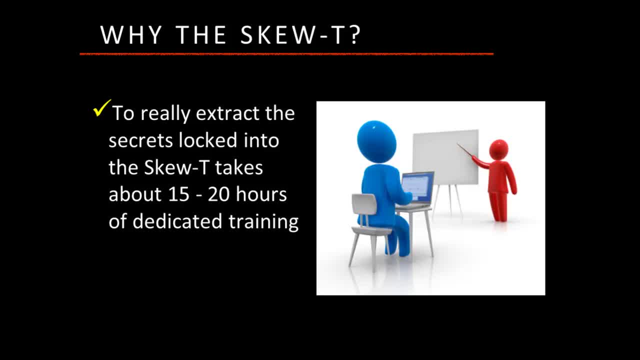 Yeah, 20 hours of dedicated one-on-one training. I've been able to do this online as well as in person And I think, overall, eventually. again, it takes a lot of practice, but eventually you get to the point of using it. It becomes natural to use it in your daily flight planning. 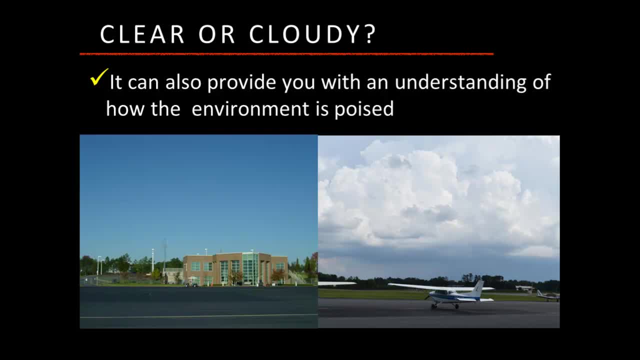 So the other aspect of it. it can really provide you an understanding of how the environment is poised. Are you going to have a clear day, like you see here on the left, or more of a cloudy, more of a convective day, as you see on the right? It also will help you determine where. 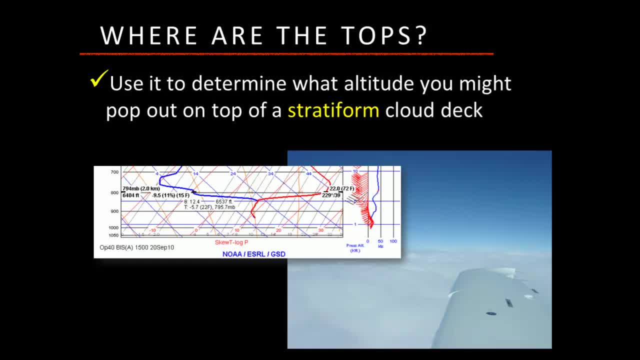 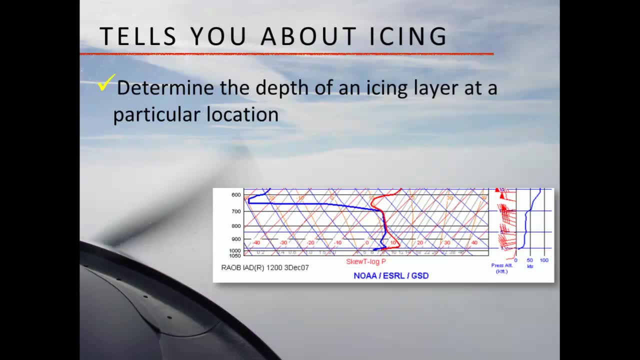 maybe the bases and the tops of a stratiform cloud deck are located, And it also tells you a lot about icing, So it gives you the indication of the depth of an icing layer at any particular location, Really helpful, especially during the wintertime, where we see. 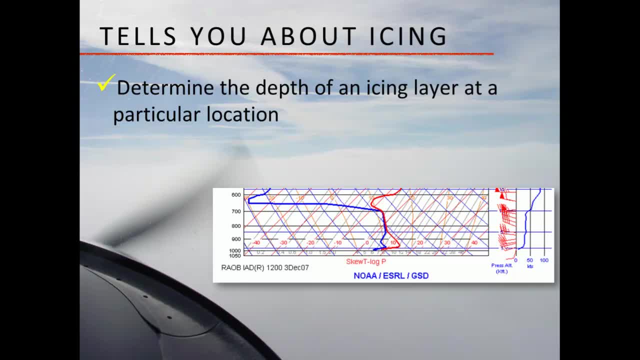 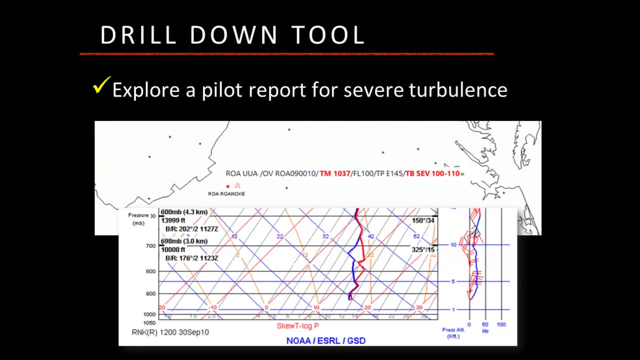 most of the icing incidents and accidents that occur. So this is a great tool to be able to drill down and determine what's happening from an icing perspective- And we'll talk about both those stratiform clouds and icing a little bit later. I really love to use this tool more than anything else to explore and drill down on things like a. 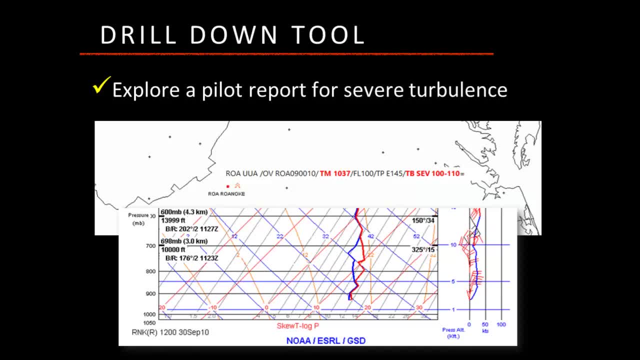 severe pilot report for turbulence. So in this particular case, I was departing out of Roanoke, Virginia, and I noticed there was a pilot report for severe turbulence at between 10 and 11,000 feet. So I pulled up the radio sun observation and took a look at it And, sure enough, I could see. 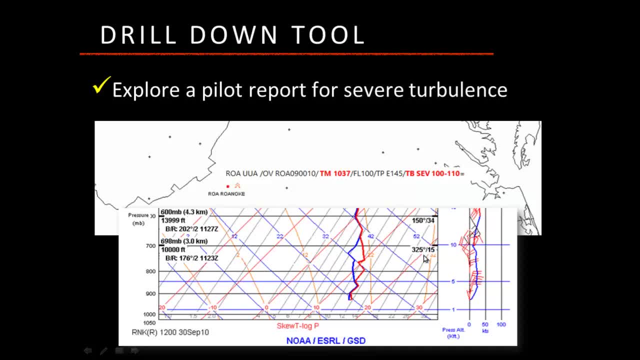 that the winds were really interesting at that altitude. So the winds are 325 degrees at 15 knots, and they increased, but they changed direction to 150 degrees at 34 knots. So what you see here is what essentially looks like a tumbleweed in the wind field, And that, along with a couple of other aspects of the 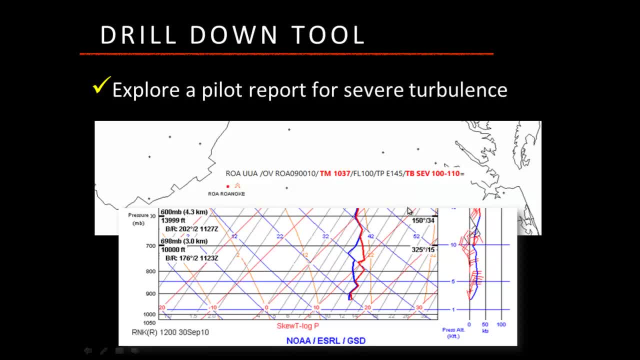 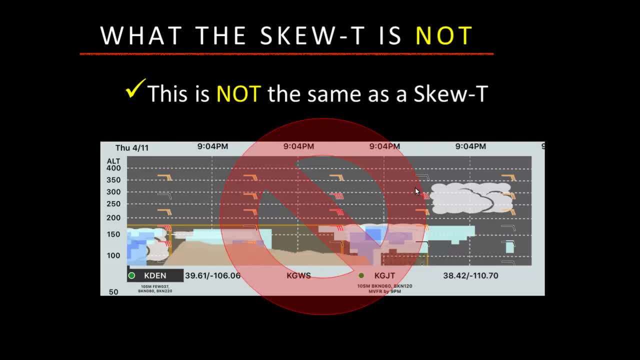